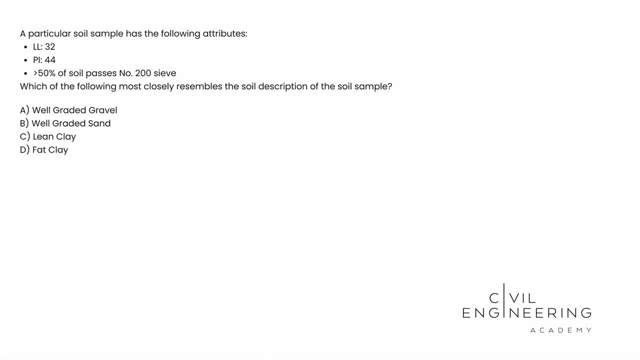 how they classify a soil type, And so right away we're looking at our options that are available to us. That's going to be the USCIS method. So that's step. number one is identify which ones we're dealing with And if we're looking for some reading material in the FE manuals at the time of 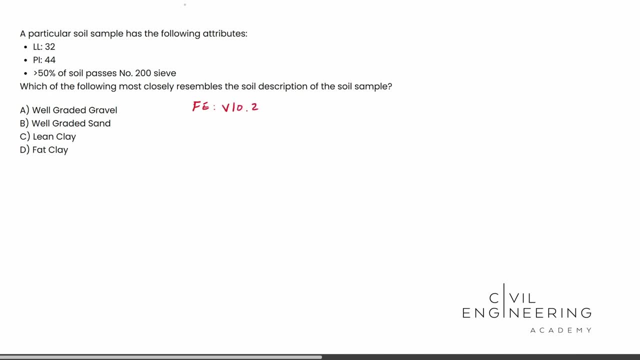 this video. it's going to be version 10.2.. We're going to be in the civil engineering section. So CIV I, L, E, N, G- I'm going to write that for short, And then we're going to be in page 267.. So page. 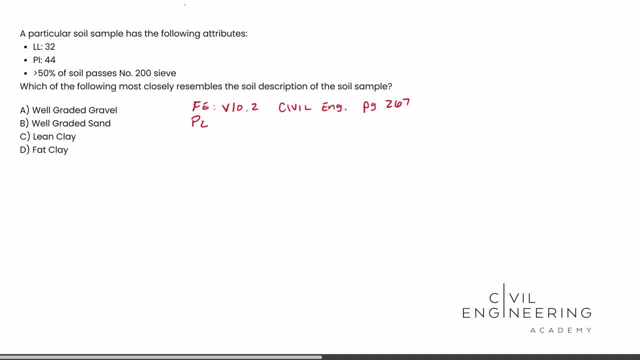 267.. And then in the PE manuals, we're going to be in version 1.1.. And this is going to be in section 3.7.2. And we're going to be in page 116.. So that's where we're looking, That's where you. 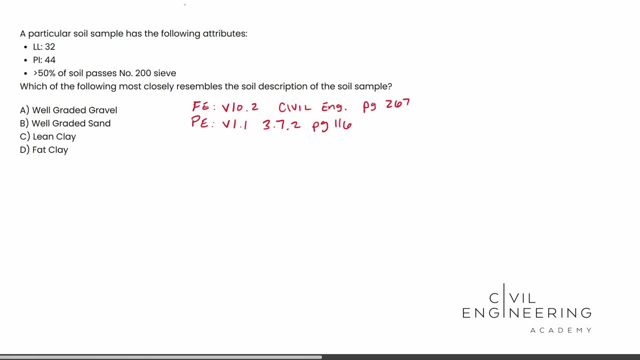 can find the classification charts, the USCIS classification charts. I'm not really sure if I can pull it over, if I can include a snip. So we're going to play it safe due to copyright issues And I'm just going to have you guys. 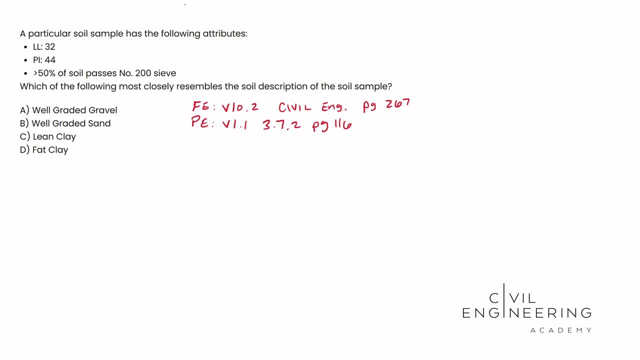 follow along with me. I'm going to try and write down the steps best I can, but it would really be good for you to pull up the manual on maybe half your screen and have this video going on the other half of the screen and just follow along, see if it makes sense to you And we'll. 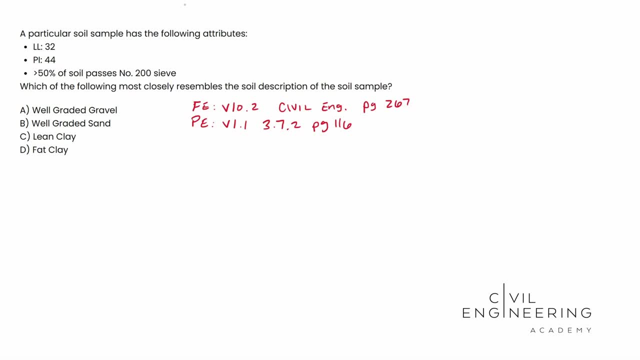 work through this problem together. Now, whenever we look at the USCIS classification chart, if you're taking the FE, you'll notice that the coarse grain soil and fine grain soil classification or difference really is on the left side of your chart, Whereas in the PE. 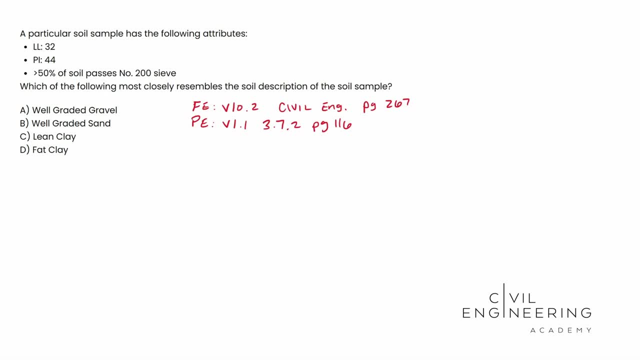 it's up top. It's on the top of your chart, but the rules still apply. I mean, it's just a different way to look at it here, but let's see. So the first classification here is 50% or more, or sorry. 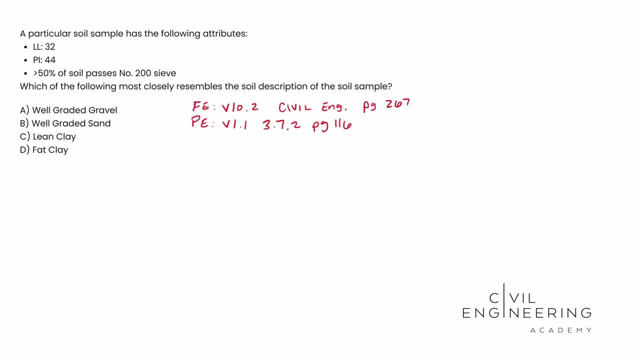 more than 50% retained in the number 200 SID. That doesn't really apply to us because we have greater than 50% of the soil passing the number 200. So don't get that mixed up. Basically, if it's, you know, if it's retained, the size is greater. 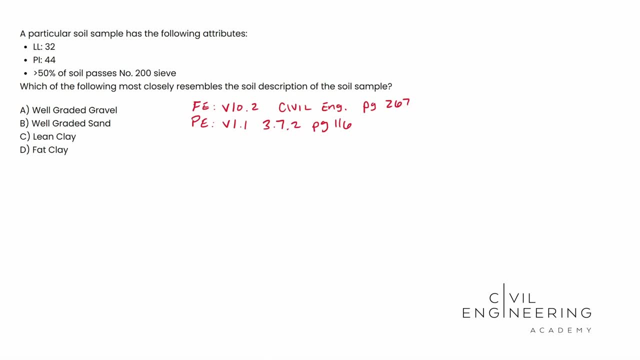 than that SID. So we're talking a number 200 SID- 0.075 millimeters. anything greater in size than a 0.05 millimeters is going to stay above it. It's going to be retained in that SID, Whereas 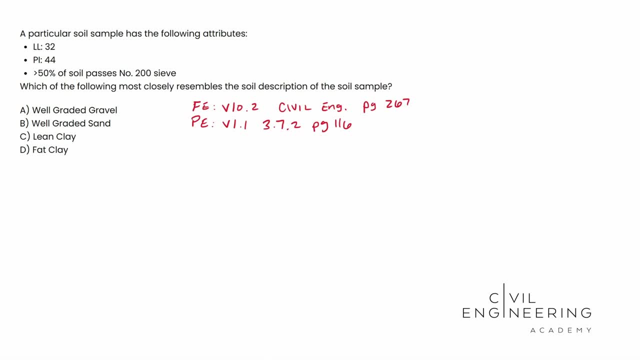 if it passes, it's smaller than 0.075 millimeters, So that we're going to be dealing with some fine stuff. And so, uh, that that's the next classification. there is fine grain, soil, silts and clays. That's what we're going to. 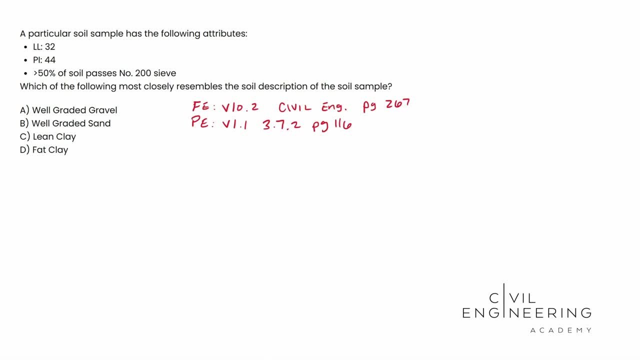 be dealing with, And so you can ignore the other half of the USCIS classification chart right. So the coarse grain soils doesn't apply to us. We're dealing with some fine stuff, silts and clays in particular. Now the the. the next requirement is the liquid limit. Is it less than or greater? 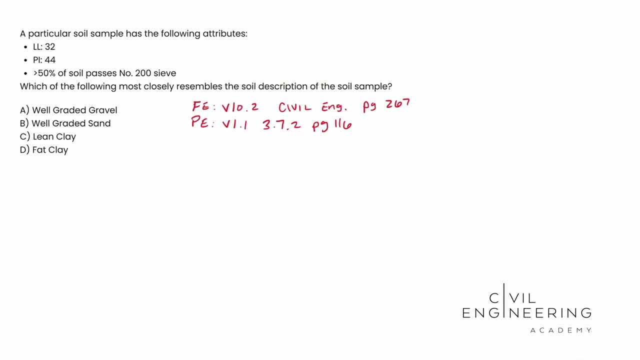 than 50? Well, in our case it's 32 less than 50. And so that means that we're dealing with, we're going to uh further, uh, filter, I guess, our um, our chart, I guess, to only include half of the fine grain soils. 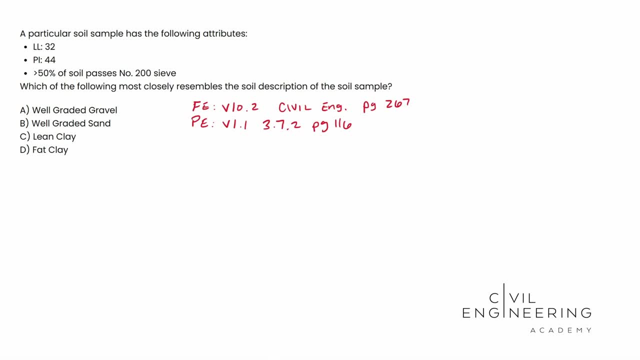 classification. So now we're talking silts and clays with the liquid limit less than 50. So that CLML or OL, so low plasticity stuff, is what we're dealing with. And so now, uh, the further classification: inorganic, organic. we don't know that, it's not given to us in the 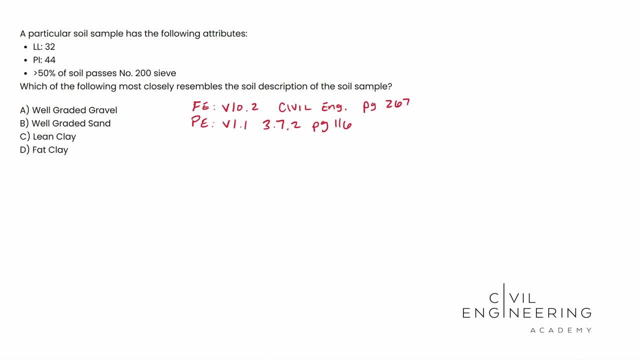 problem. And then we're kind of given like, uh, some weird stuff, So the PI: it needs to be greater than seven and plots on or above the A line, or so that will give us the CL, the lean clay, or uh, PI needs to be less than four or plots below the A line. That's the ML. 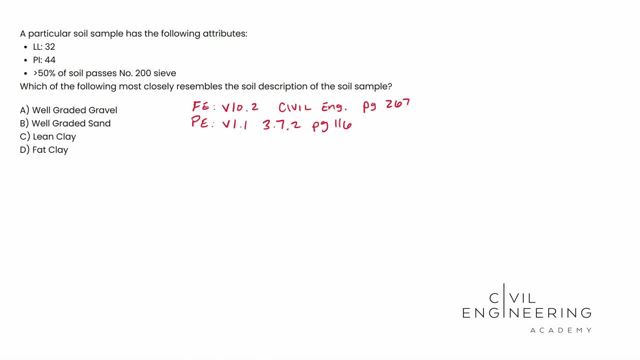 the silt. low plasticity silt- That's what that L means, by the way. Uh, but that's not even an answer in our problem. So you can go ahead and ignore that, but I'm going to go ahead and show. 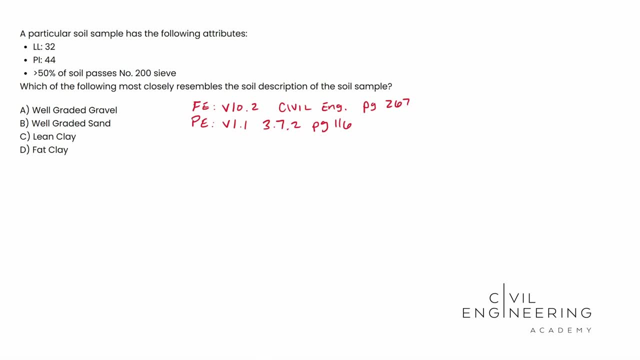 you or walk you through how to uh, how to solve that uh on the chart. So then the next cloth, the next qualification, as if it's an organic, low plasticity, uh, clay or silt, right, Well, that's also again.